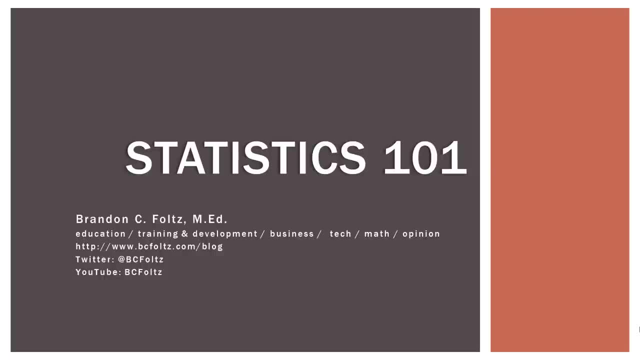 anything but my love of learning, So feel free to follow me here on YouTube and or on Twitter. That way, when I upload a new video, you know about it. And on the topic of the video: if you like it, please give it a thumbs up And, on the flip side, if you think there is something. 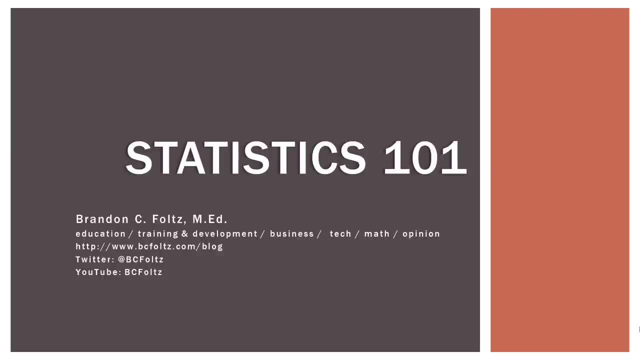 I can do better. leave a constructive comment below the video. I will try to incorporate that into future ones. And finally, just keep in mind that these videos are geared towards individuals who are relatively new to stats. So I'm just going over the basic concepts and I will be doing so. 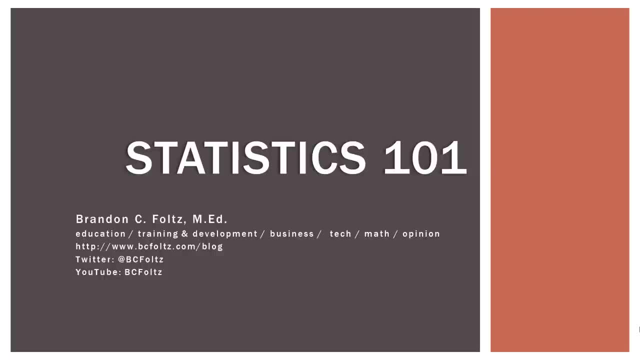 in a very slow, deliberate manner. Not only do I want you to understand what's going on, but also why. So, all that being said, let's go ahead and dive right in. So in this video, we're going to continue our discussion on probability distributions. 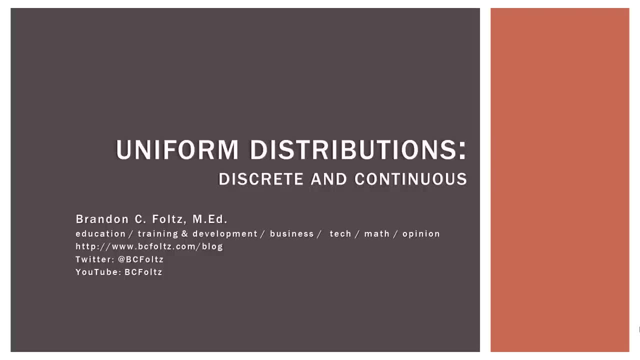 Now I've done several videos on other distributions, like the binomial distribution and the Poisson distribution. In this video we're going to look at what are called uniform distributions or rectangle distributions, And that's because they're shaped like a rectangle. 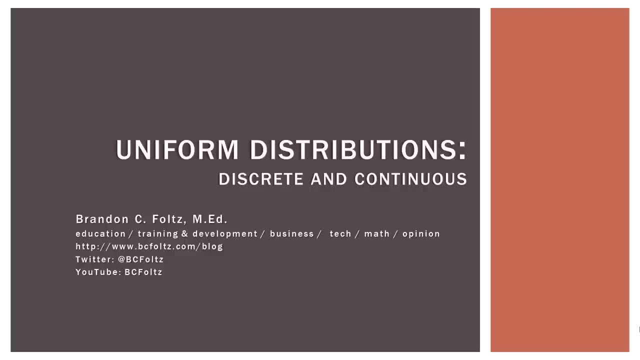 And what this will do is it will lead us into the next series of videos where we talk about the normal curve, the normal distribution, But we get there through this idea of uniform distributions and, taken to certain limits, when we talk about continuous data. 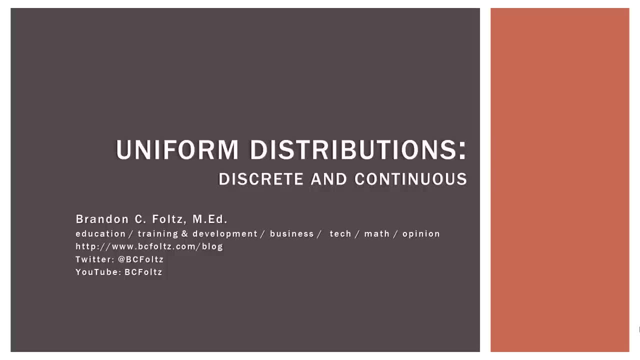 But I don't want to get ahead of myself. So we're going to talk about uniform distributions, both discrete uniform distributions and continuous uniform distributions. So let's go ahead and get started Now. what do these two events or processes have in common? 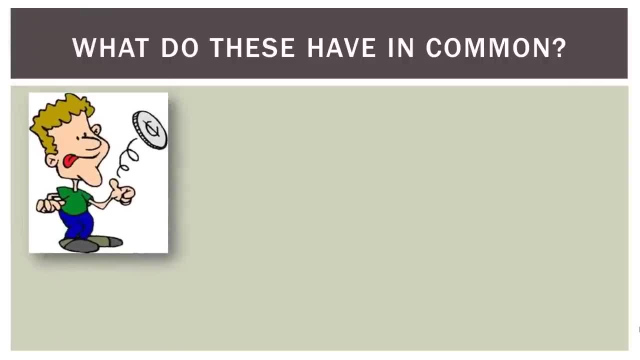 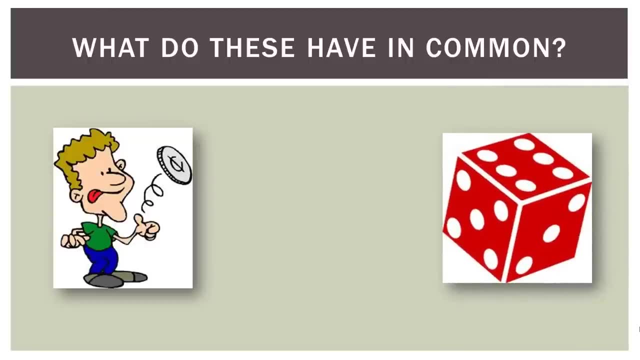 A coin flip and the roll of a die. So what do these have in common? Think about it for a second. Well, they both have a fixed number of outcomes. So the coin flip has two outcomes: heads or tails. That's it. 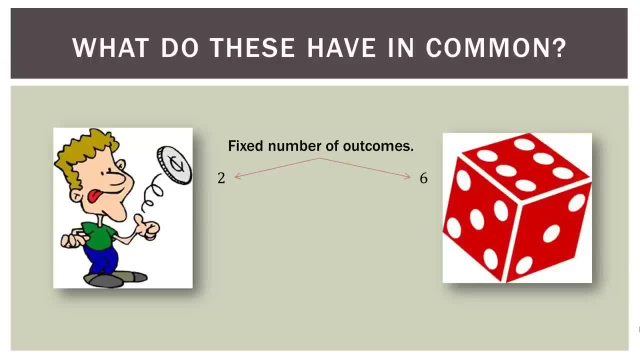 The die roll has a fixed number of outcomes. So the coin flip has two outcomes: heads or tails. That's it. My roll has six outcomes: The numbers one, two, three, four, five or six. So they both have a fixed number of outcomes. 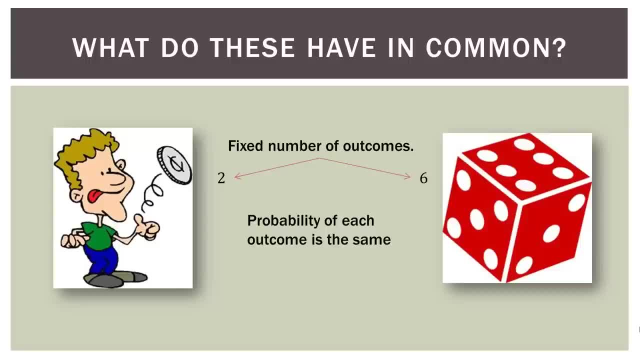 Also, assuming they are both fair, the probability of each outcome is the same. So, for a coin flip, the probability of heads is one half. the probability of tails is one half. So the same probability for each outcome. Now, how about the die? 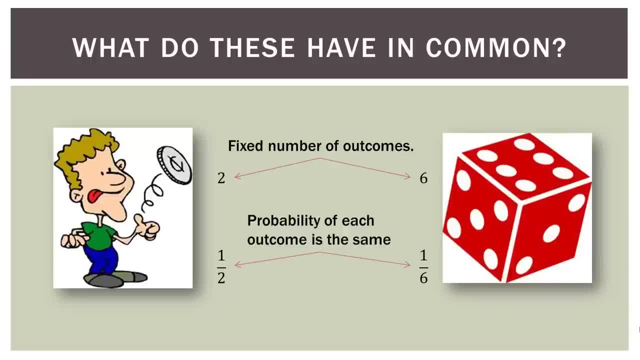 Well, the probability of any number being rolled is one sixth. There are six numbers on the die. They all have the same probability of coming up. Therefore, the probability of each outcome on a die roll is one sixth, And this is the basis of what we're gonna talk about. 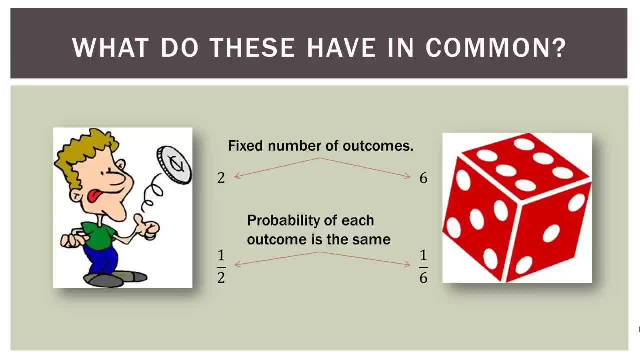 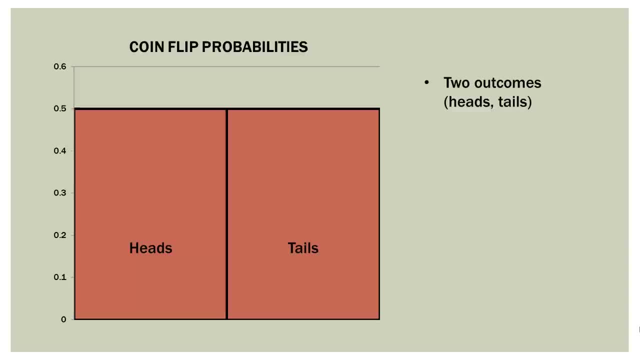 in this video. So just think about these two things as we proceed. Let's look at our coin flip. Well, it has two outcomes: heads or tails. The probability of each outcome is the same, And that outcome or the probability is one half or 0.5. 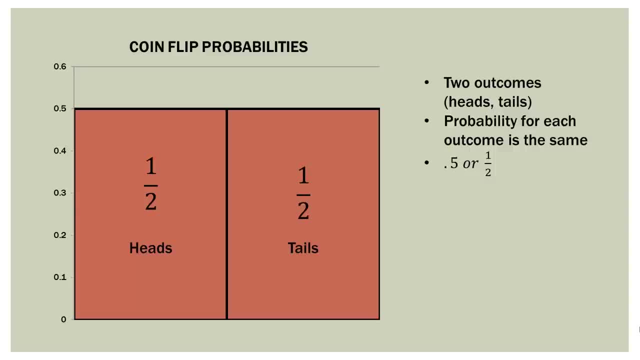 So if we graph that, we can see that for heads we have a probability of one half, which is 0.5.. If you see the Y axis there on the left, it goes up to 0.5.. And for tails it's also the same. 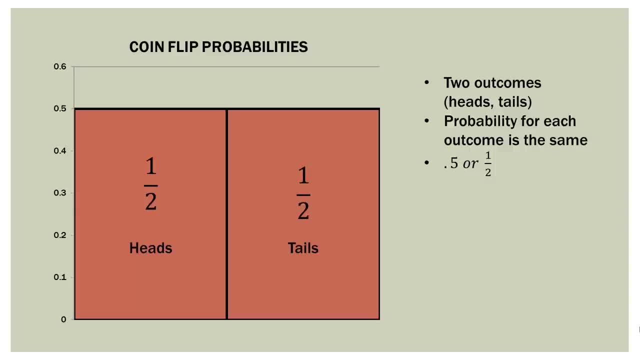 Now note that: what is one half plus one half, or 0.5 plus .5?? Well, it's one. So we know already that the probability is right, Palestine at one-half, that the probabilities have to add up to one. 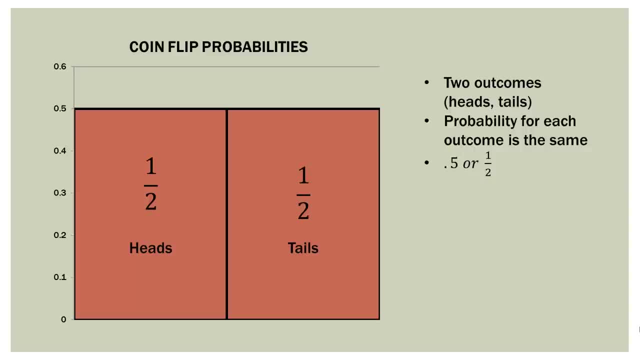 which is a very common theme we've talked about in other probability distributions. Now we call this a uniform, discrete probability distribution. Well, what makes it uniform? That's because the probability of each outcome is the same. The top is flat, it's straight across. 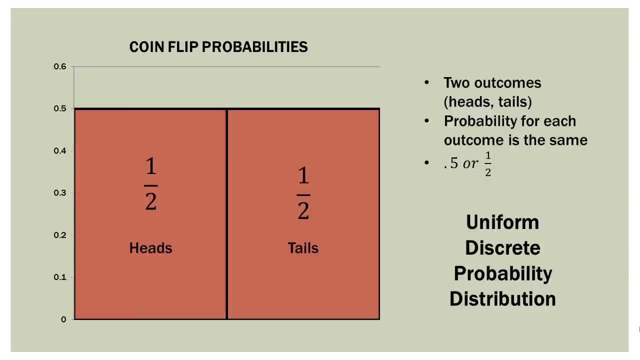 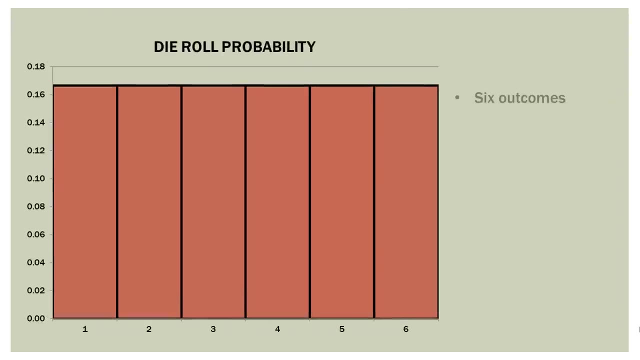 And in this case it's discrete because a coin flip can either have two outcomes, heads or tails. So a uniform, discrete probability distribution for a coin flip looks like this: Now, how about rolling the die? Six outcomes: They can be one, two, three, four, five or six. 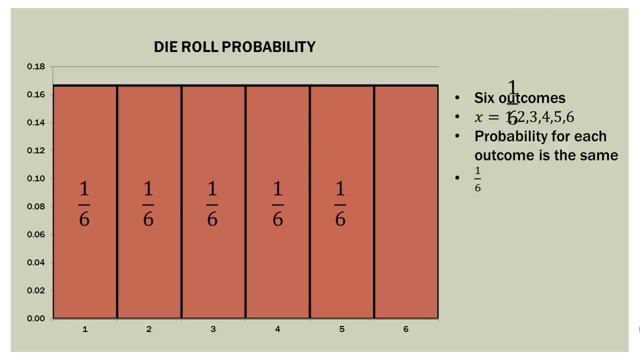 The probability for each outcome is the same. So for a one it's 1 6th, for a two it's 1: 6th, a three is 1 6th, et cetera, And you can see that 1 6th plus 1 6th. 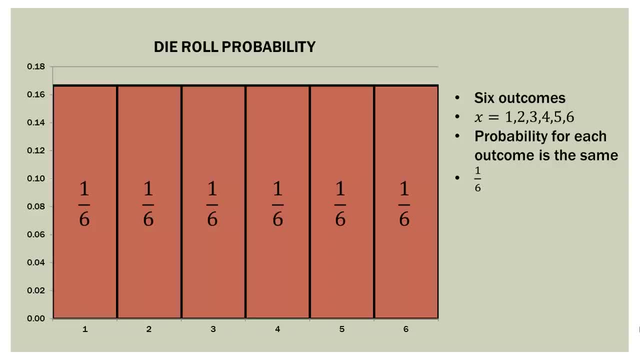 plus 1, 6th plus 1, 6th and on and on, is 6 over 6, which equals one. So this is also a uniform, discrete probability distribution. It's uniform because the probability of each outcome is the same. 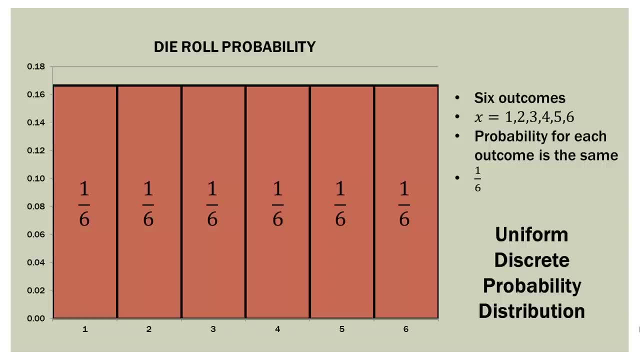 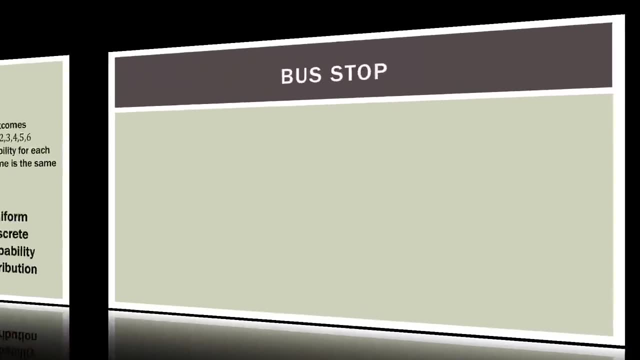 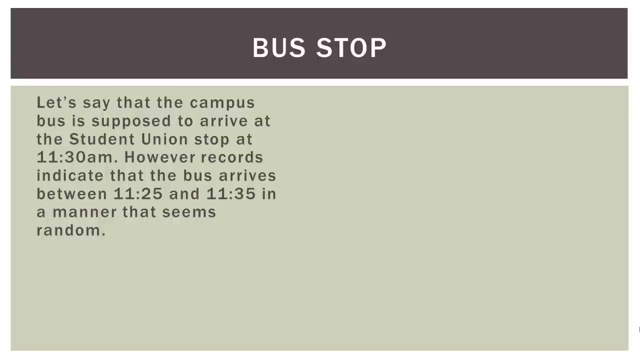 You can see there it's about .167 or so. It's flat across the top and it's the same for each outcome. Now let's talk about maybe a more real world situation. Let's say that the campus bus is supposed to arrive at the student union stop. 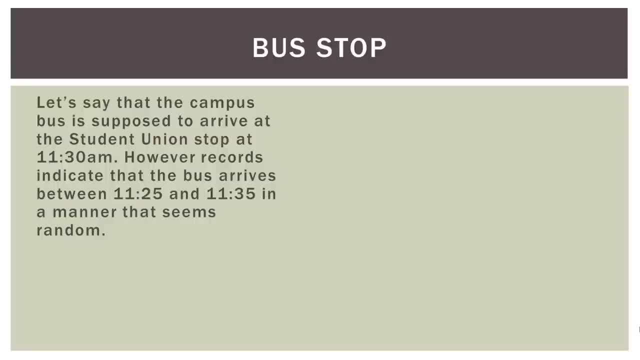 at 11.30 am. However, those of us who ride campus buses, a lot records indicate that the bus arrives between 11.25 and 11.35 in a manner that seems random. So the bus seems to arrive between 11.25 to 11.35. somewhat randomly. There's no time around which it seems to gravitate, So we can think of that as the bus arrival time during any one minute interval is just as likely as the next one minute interval. So from like 11.25 to 11.25.59,. 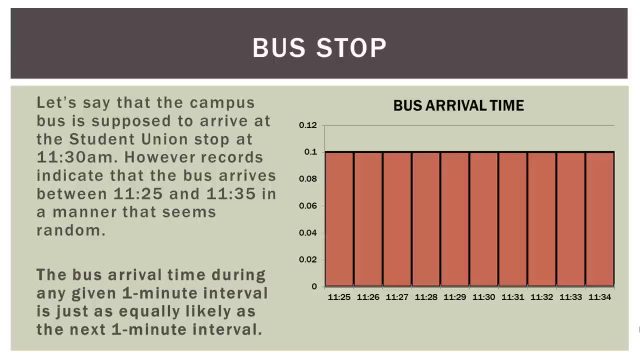 the probability of the bus arriving during that minute is the same as the next minute, which is the same as the next minute, and so forth across that 10 minute span. So we've taken our 10 minute interval and sort of chopped it up. 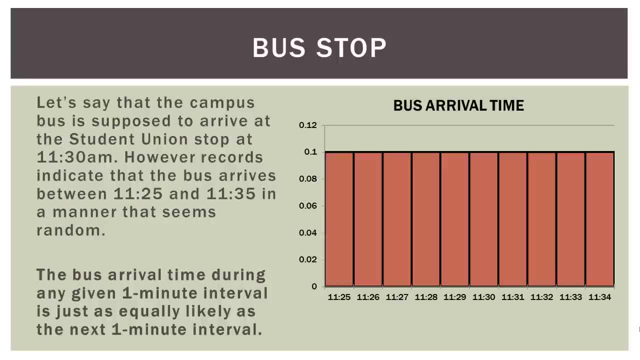 into one minute time spans, And the probability of the bus arriving in any one of those time spans is the same. So here again we have a uniform distribution. You can see that the height is 0.1, which of course is 1.10, and it's straight across. 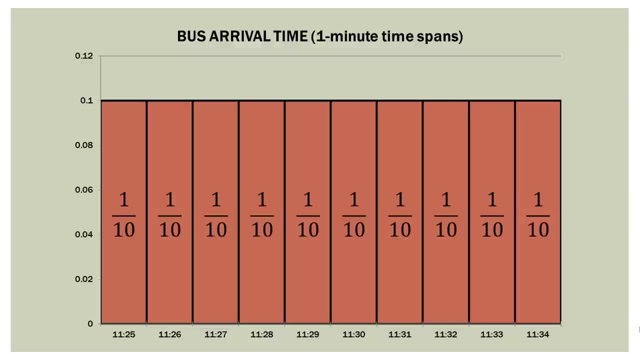 So, again, each outcome is 1.10. and if we were to add up all those probabilities, what would it be? Well, it would be one. So this is just the third example of a discrete uniform probability distribution. so you can visualize it in your mind what it looks like. 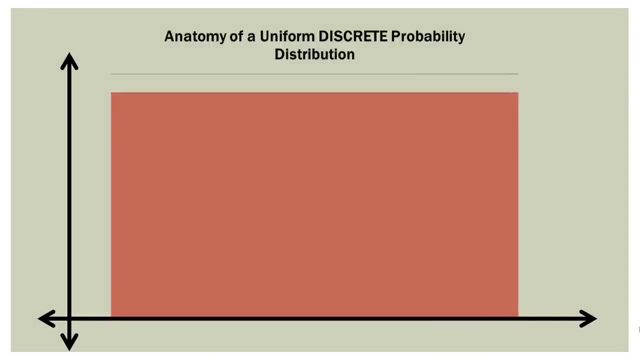 Now let's talk about the anatomy of a uniform, discrete probability distribution. So if we look at just the shape here, of course we have our axes, the x-axis on the bottom and the y-axis, the vertical axis. Well, what shape is this? 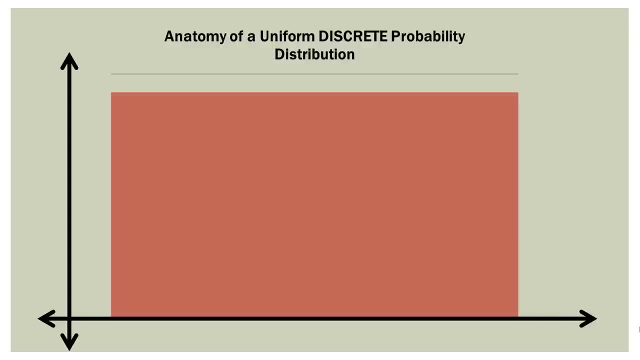 Well, it's obviously a rectangle, So sometimes these are called rectangle distributions or rectangle probabilities, but really the real way to think of them is uniform probability distributions, So probabilities on the left-hand side, on the vertical axis, and on the bottom we have the number of outcomes. 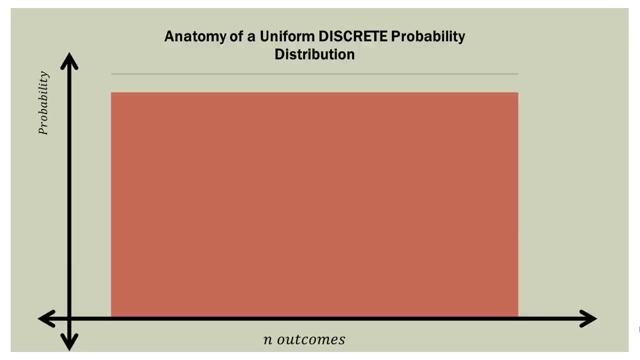 So remember, for our coin flip, we had two outcomes. for our die roll, we had six. for our bus stop, we had 10.. We know that the total area of this rectangle has to equal one. The probabilities always add up to one. 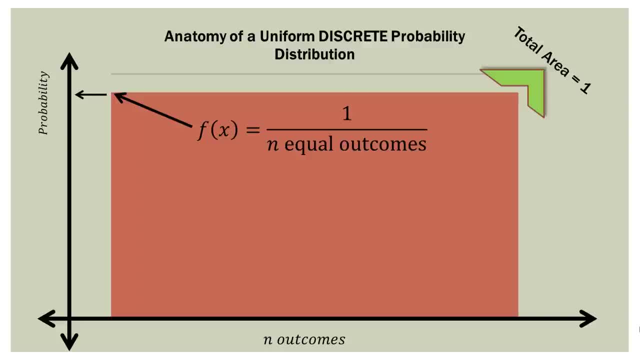 Now we have this probability density function, and don't freak out, this is what we've been doing the whole time. So the height of the rectangle is just one: the overall probability of one divided by the number of outcomes we have, And this should sort of make sense. 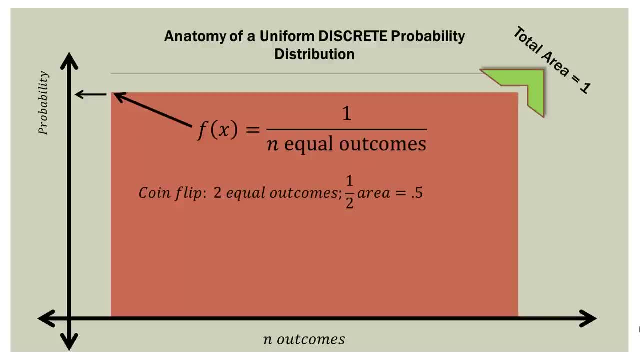 because remember, for the coin flip, we had two equal outcomes, so each outcome had one half the area, which was .5, and we had two bars in our rectangle And the die roll had six equal outcomes, so each one was one sixth the area. 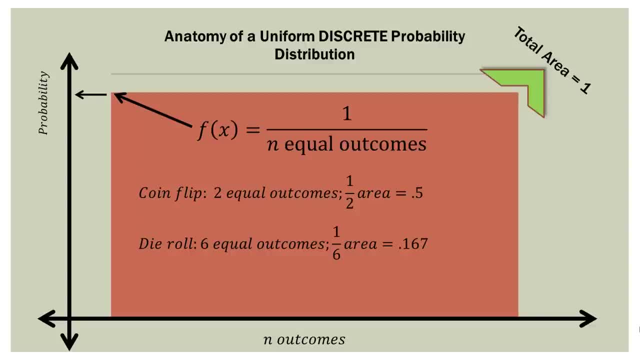 or .167, because our rectangle was split into six even bars For our bus stop. For our bus stop, it had 10 equal outcomes, So each one was one-tenth the area or 0.1.. And it was 10 equal bars in the probability area. 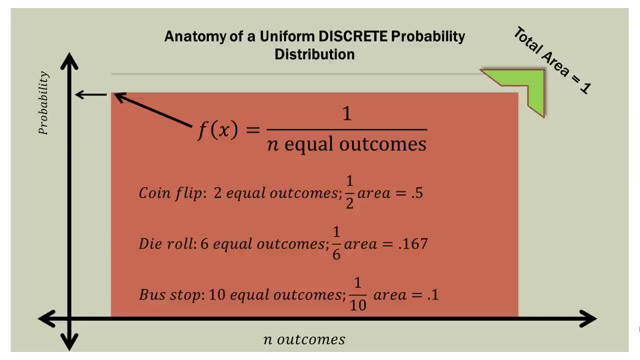 So you can see that this probability density function, this f of x for a discrete probability distribution, is just 1 divided by the number of equal outcomes we have. That's it. There's nothing more complicated than that. And that is the height of the bars. 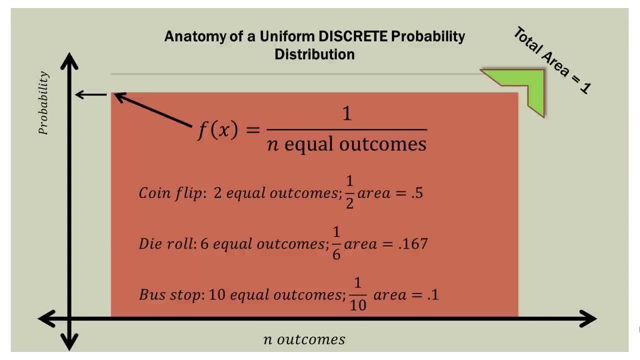 Now, as you can see, as the denominator gets larger. so 1 half is 0.5,, 1 over 6 is 0.167,, 1 over 10 is 0.1, of course, the height of the bars is getting smaller and smaller and smaller and smaller. 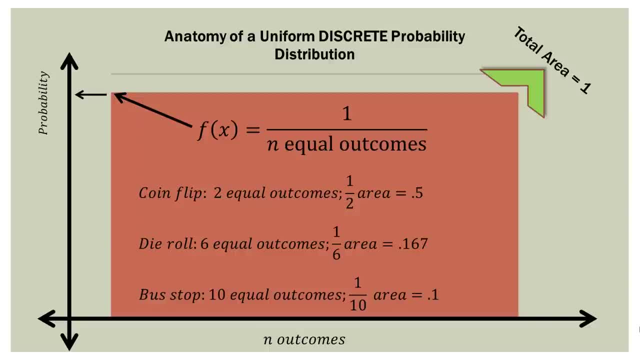 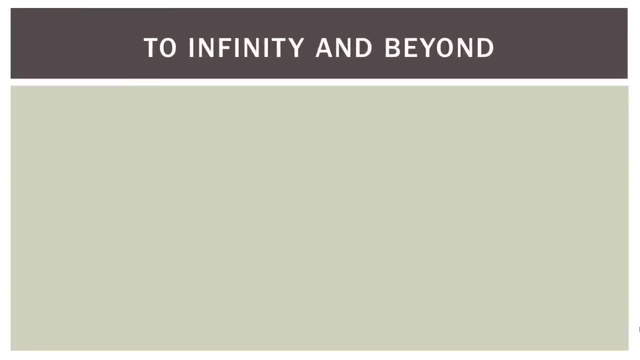 as the number of outcomes increases, And that's going to be a pattern we talk about here in a minute because it's very important. So let's talk about this to infinity and beyond. Well, what do I mean by that? Well, what we can see is that the uniform probability distribution of each discrete outcome 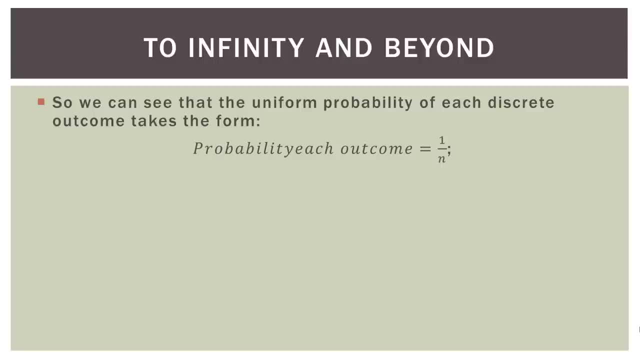 takes the form of what we just talked about. The probability of each outcome is 1 over n, So 1 over 2 for the die roll, 1 over 6,, I'm sorry, 1 over 2 for the coin flip. 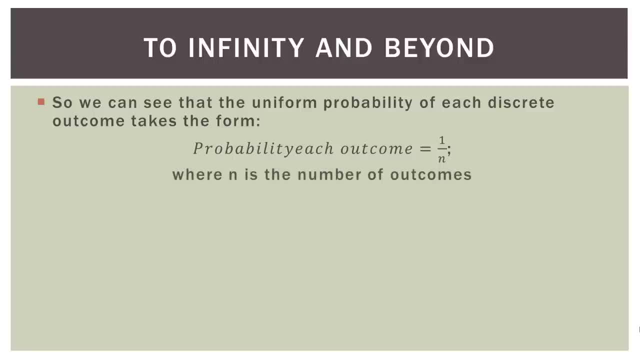 1 over 6 for the die roll and 1 over 10 for the bus stop, where n is the number of outcomes. But think about data such as temperature, Distance, income mass. that can be measured very precisely to several decimal points. 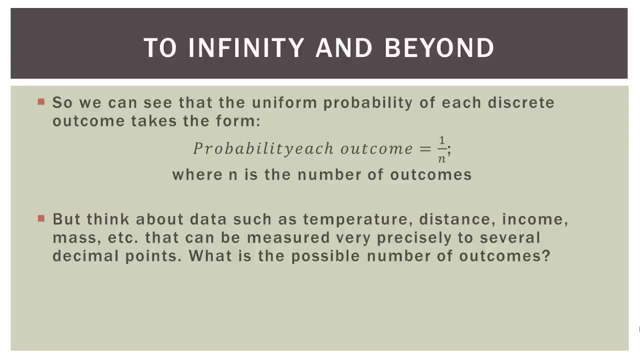 So think about the very finely, the very high precision scales you would use in a chemistry lab that may have 3 or 4 decimal points when you make the measurement of whatever mass you're doing. How many possible number of outcomes would be there? 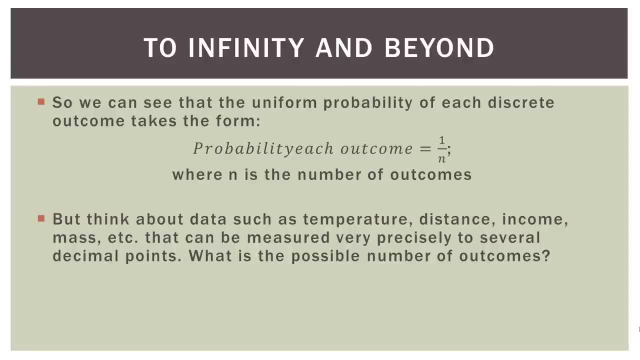 I mean, think about it: 1,, 2,, 3,, 4,, 5 decimal places, That is a crazy number of specific outcomes. So what's the possible number of outcomes as n becomes very large? Infinite, Infinite. 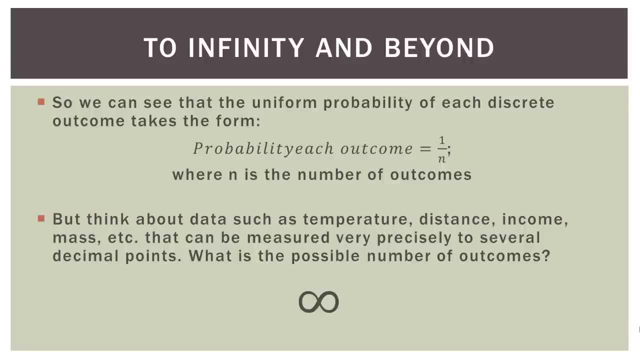 Because, remember, the coin flip is just 1 over 2.. That's it. Die roll 1 over 6.. That's it. But if I take, you know, a measurement of sodium bicarbonate and I place it on a cube, 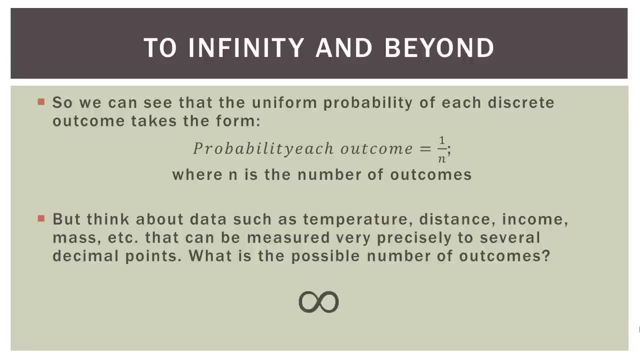 and I put it on a scale, it might be 2.3456 grams. Am I going to have an outcome for 2.567 grams, 2.5678 grams, 2.5679 grams? Am I going to have an outcome for each one of those? 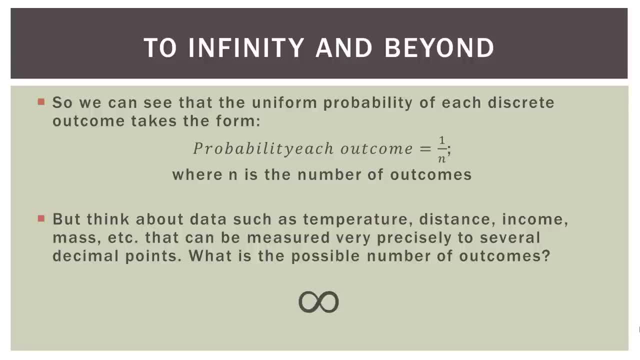 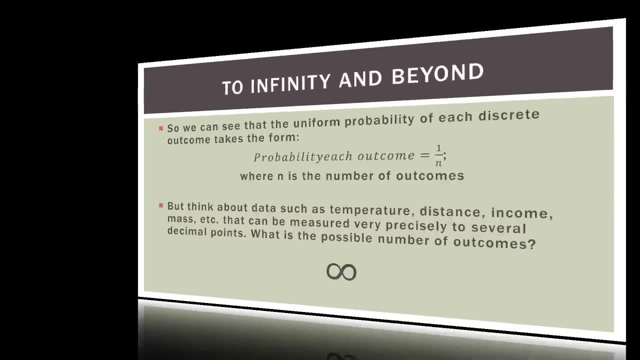 No, Okay, because that's almost an infinite number of outcomes, And that's the idea of continuous data we'll talk about here in a second. So, when dealing with this type of data, we are left with the following data: We are left with the following odd equation: 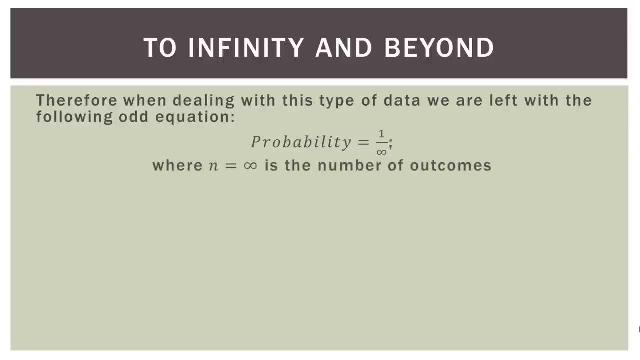 The probability is 1 over infinity. Where n is basically infinity is the number of outcomes. Well, guess what? 1 divided by infinity is treated as 0.. 0.. So think of a bar chart where the height of an infinite number of bars 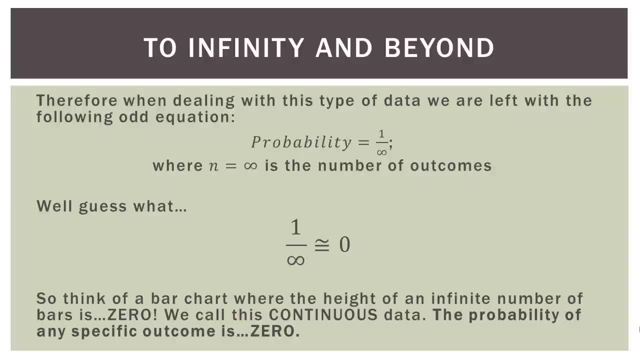 their height is 0.. That seems kind of crazy, I know, But that's what happens As n becomes very, very large. as the number of discrete outcomes goes towards infinity, the probability of each one is basically 0. And we call this continuous data. 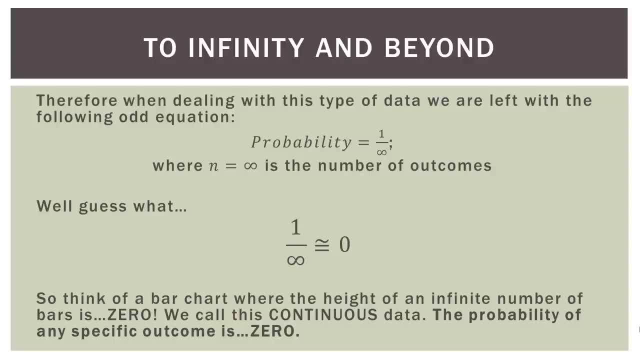 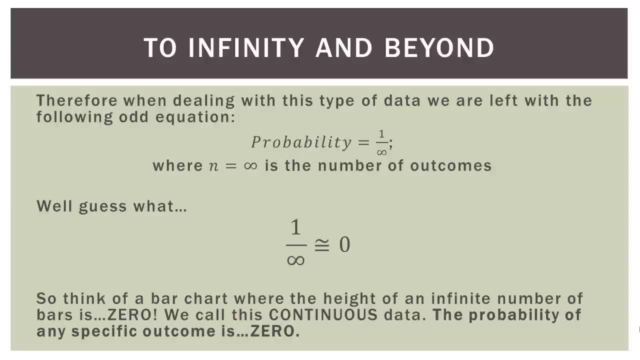 1 sixth, 1 sixth. The outcome of the bar chart is zero. bus arriving between 1127 and 1128 was one-tenth. But the probability of putting my potassium chloride, or whatever I'm measuring, on a scale and it coming up exactly 2.5678 grams is nearly infinite. 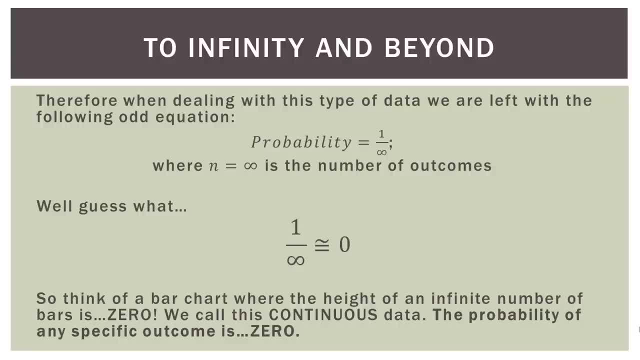 There are an infinite number of possibilities because of the precision of the measurement device, But just think of it. the probability of any individual outcome in a continuous distribution or continuous measurement is basically zero, And that's what makes continuous data what it is Now. don't freak out. 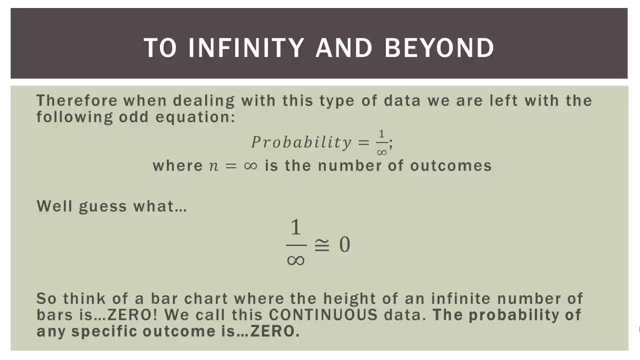 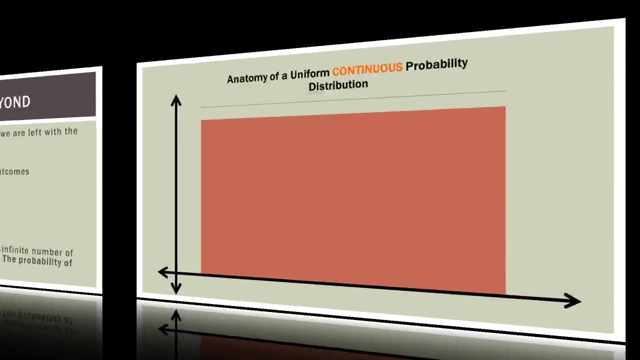 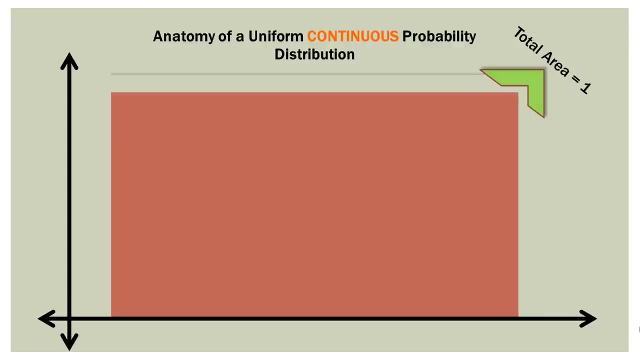 because we're gonna do several examples. but just keep in mind, as n becomes closer to infinity, the probability of each outcome is basically zero. So talk about the anatomy of a continuous probability distribution As opposed to a discrete one. Well, the shape is still the same. 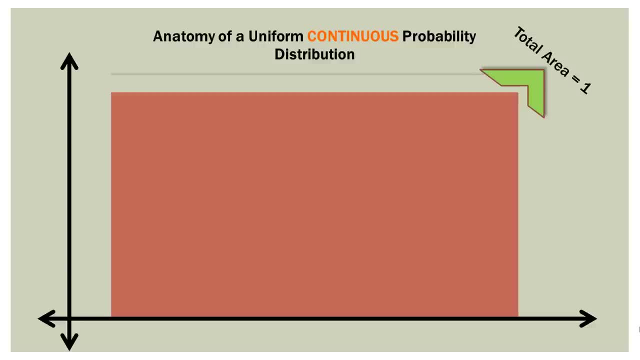 We have our axes. The total area is still one. What we do is we sort of label each end of the distribution: A and B. That just marks the end of our distribution. Now, anything to the left of A is zero. Anything to the right of B is zero. 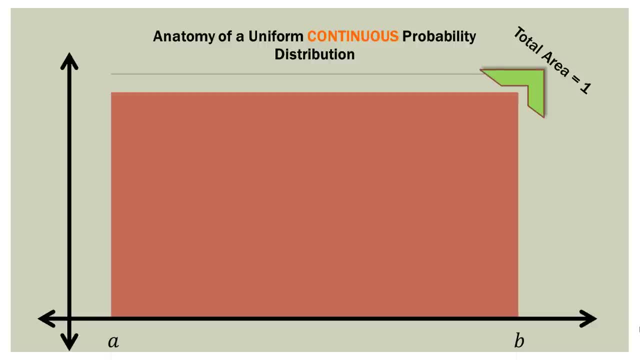 So all of our probability is between A and B. Now the distance from A to B is the width of our distribution. literally It's the width of our probability distribution. So how can we represent that algebraically? Well, it's B minus A. 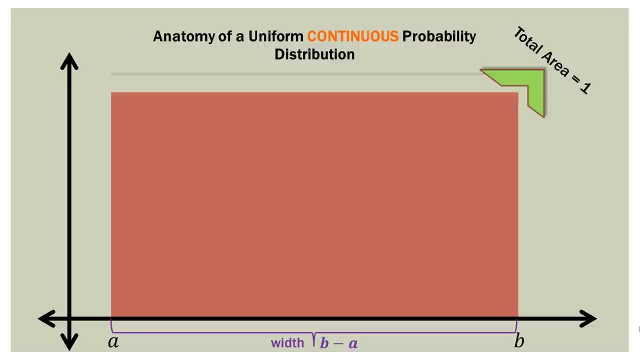 The distance from the vertical axis to B minus the distance from the vertical axis to A leaves us with the width of our rectangle. So the width of our probability distribution is B minus A. Now we know from elementary school that the area of a rectangle like this 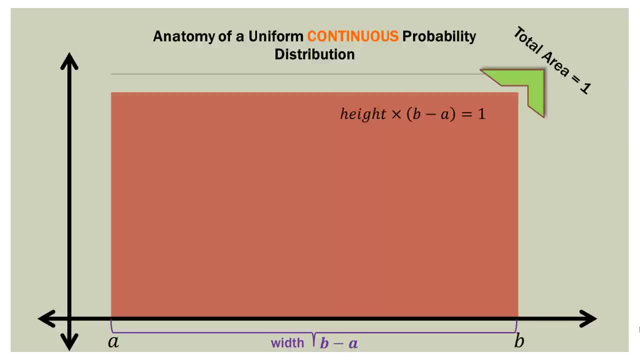 is the height times the width. Well, the height, we're not sure yet. That's what we're gonna find out, But we know the width is now B minus A And we multiply those together, it has to give us an area of one. 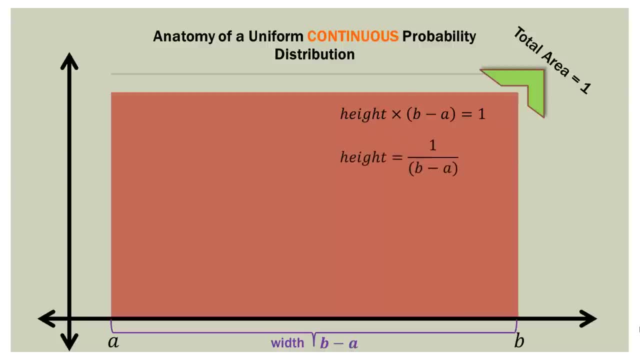 So, with a little bit of algebraic manipulation, the height that we don't know yet is one divided by B. So the height that we don't know yet is one divided by B. So the height that we don't know yet is one divided by B minus A. 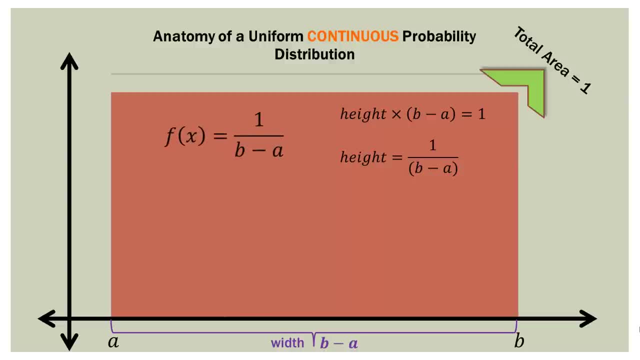 That's just simple, straight algebra. Now we call this our probability density function. So the height of our rectangle is one minus one divided by B minus A, And of course we will get B minus A in the problem we are given. So again, it's just the area of a rectangle. 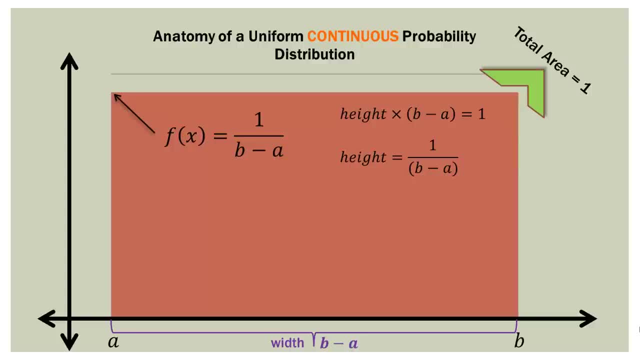 We know two things and we're gonna use those two things to find the height, which we won't know until we get the problem. So, instead of the probability of any specific outcome, which is zero for continuous data, we can only find the probability over a specified interval. 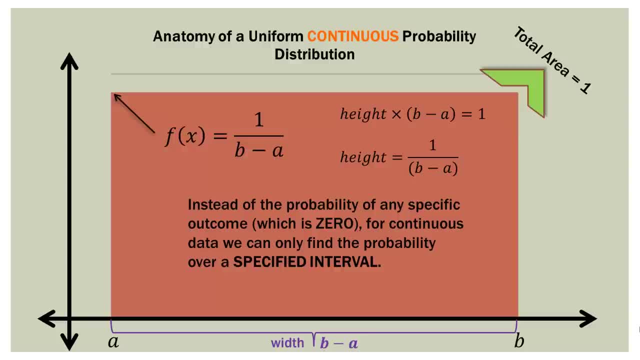 So, from A to B, the probability of any specific number in there is zero. All we can do is we can, because what we're doing basically is we're we're taking this rectangle and we are chopping it up, and we are chopping it up. 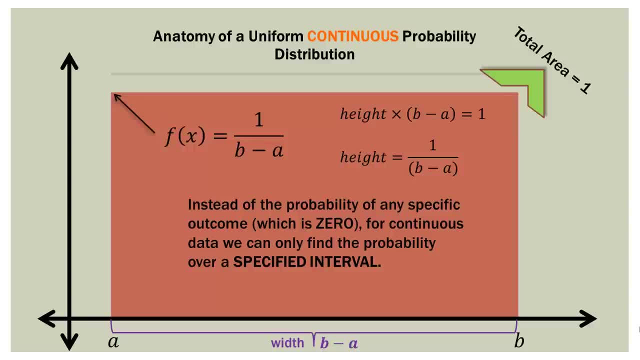 and we are chopping it up into an infinite number of bars. That's what we're really doing. So any one of them has a probability of zero. So what we can do- we can only do- is find the probability of an interval. 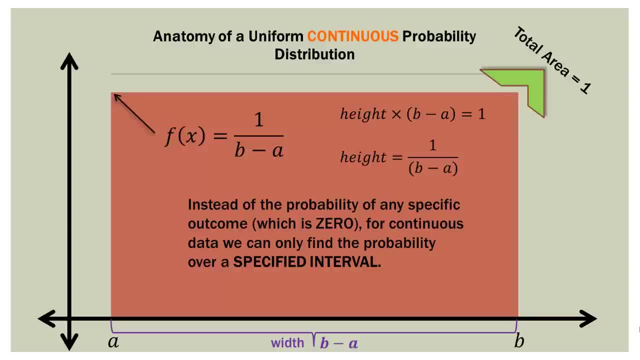 or a section of this rectangle, which we're gonna do. Now a few other things before we dive into our problem. The expected value of our continuous probability distribution is merely just a midpoint between A and B, So A plus B divided by two. 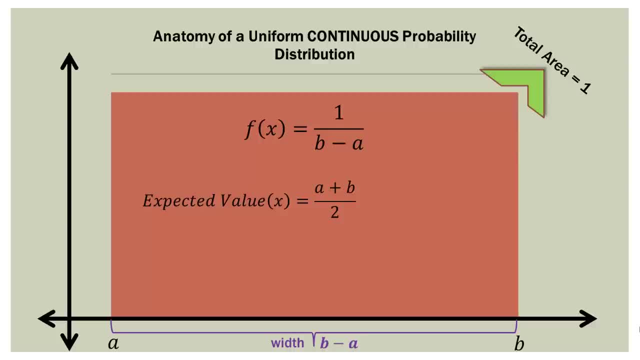 that would give us our expected value, or you can think of it as the mean, if you would like, The variance, just like any distribution can have a variance which is sigma, squared is just B minus A, all squared divided by 12.. 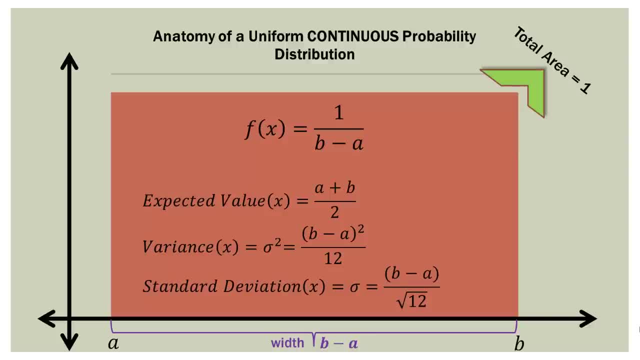 And the standard deviation again is just the square root of all that. So B minus A divided by the square root of 12.. So if we're gonna find out the expected value or the mean, the variance and standard deviation of the continuous probability distribution, 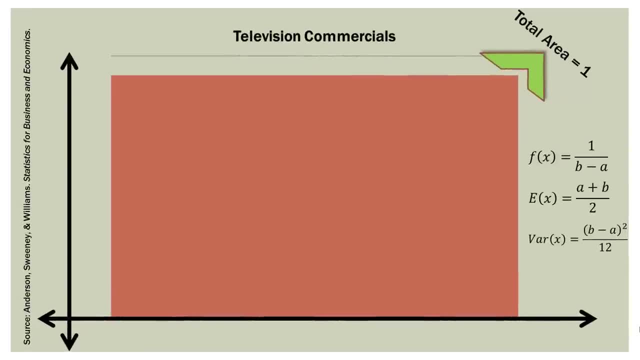 that's how you would do that. So here's our first example. On average, 30 minute TV shows have 22 minutes of actual program. We love those commercials, don't we? So let's assume the probability distribution for number of minutes of actual program. 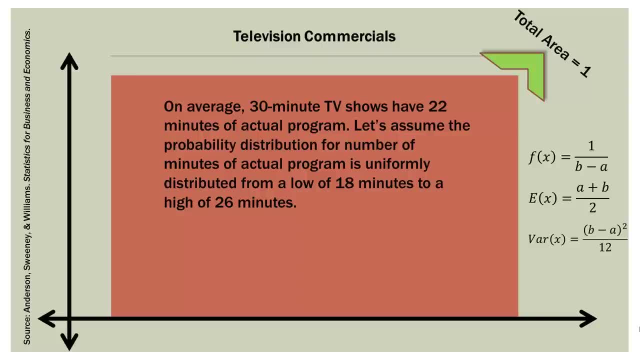 is uniformly distributed from a low of 18 minutes to a high of 26 minutes. Okay, So, on average during a 30 minute TV sitcom there's 22 minutes of actual show, But it's not always gonna be 22 minutes. 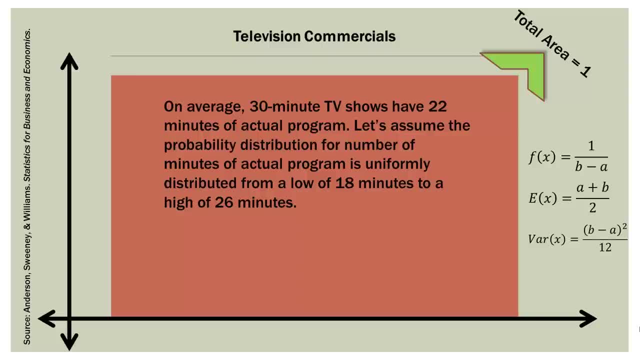 it can vary a bit, But we found that it's uniformly distributed from a low of 18 minutes to a high of 26.. So in this case, A is 18, that's our low end. 26 is B. 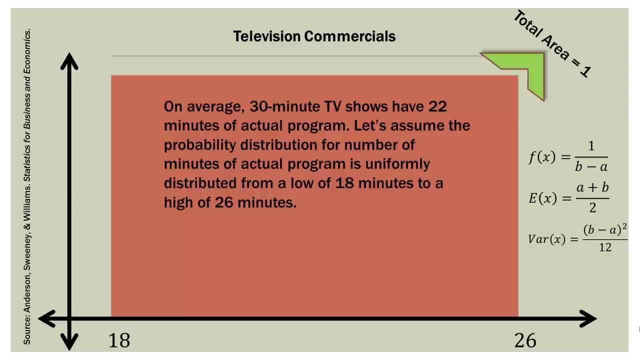 that's our high end, So we can set up A and B to represent the end points of our distribution. Now if we wanna find the probability density function, the F of X, which is the height of our rectangle here, we just go ahead and use our formula. 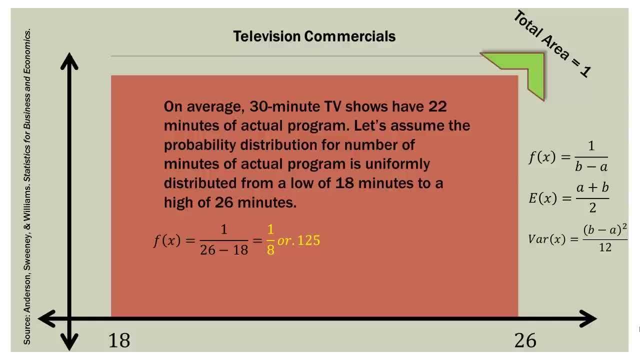 So one divided by 26,, which is B minus 18,, which was A. so one over B minus A equals one eighth or .125.. Therefore, the height of our overall rectangle is one eighth or .125.. 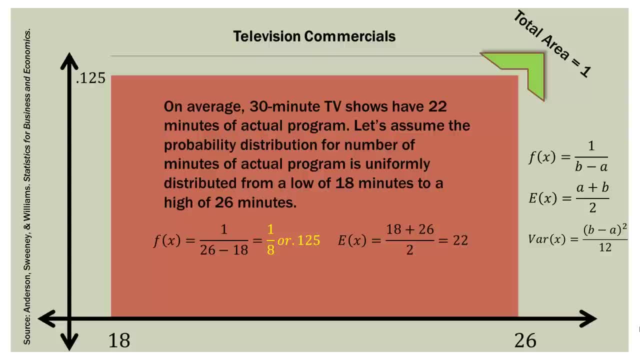 Our expected value- or we can think of it as our mean- is 22,, and of course that's given to us in the actual problem. Our variance, if we're interested, is 5.33, and our standard deviation is 2.31.. 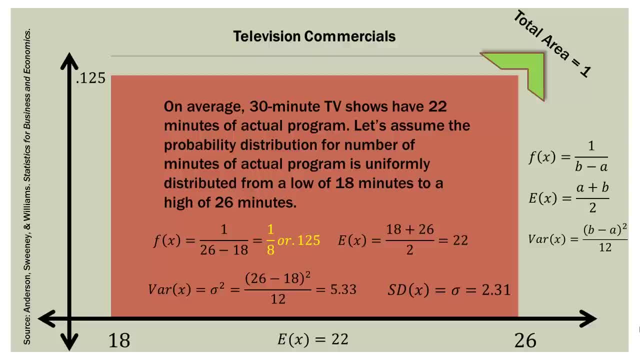 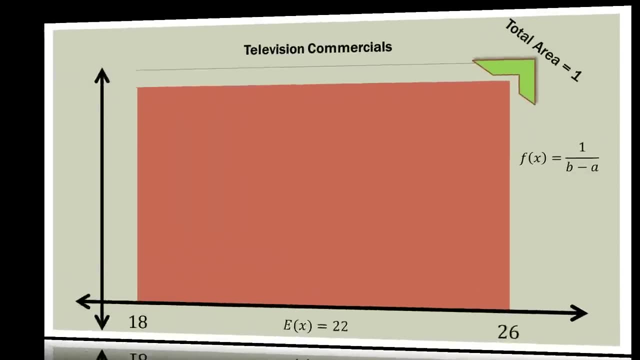 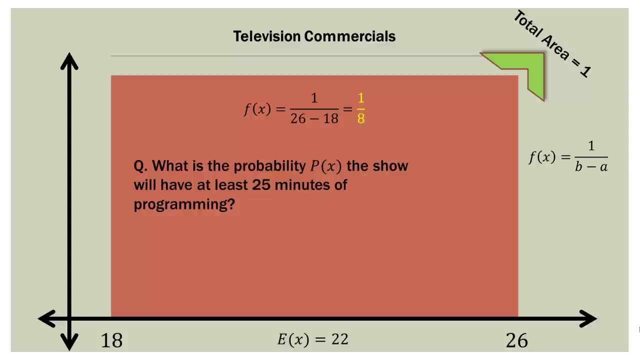 So some problems may ask you the variance and standard deviation, some may not, but they're very simple, very easy to calculate. So, using the same problem, we're gonna go ahead and put our density function up there. So remember, the height of this rectangle is one eighth. 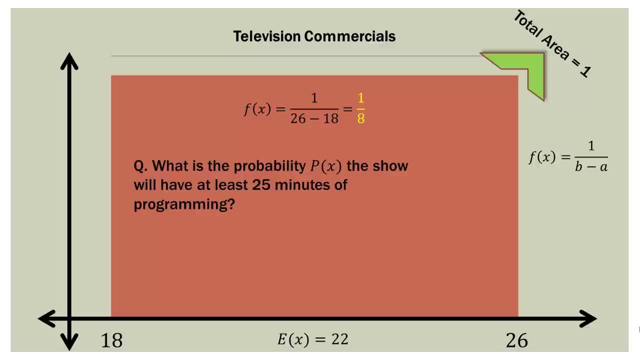 So here's a question: What is the probability P of X that the show will have at least 25 minutes of programming? So at least 25 minutes. So we're interested in the part of this distribution that is 25 minutes or more. 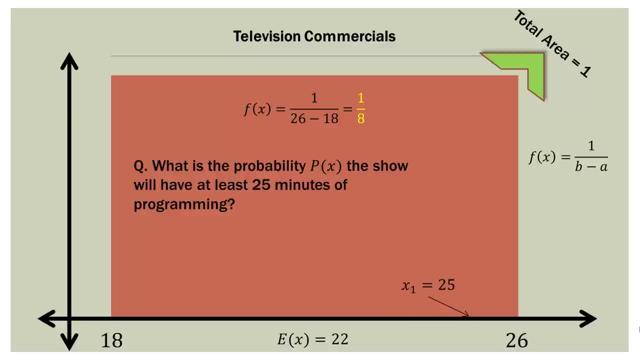 So 25 minutes is down here on the right, about right there, and of course we can only go as high as 26.. So we sort of have this section between 25 and 26 we're interested in. So we wanna know the area of this blue part. 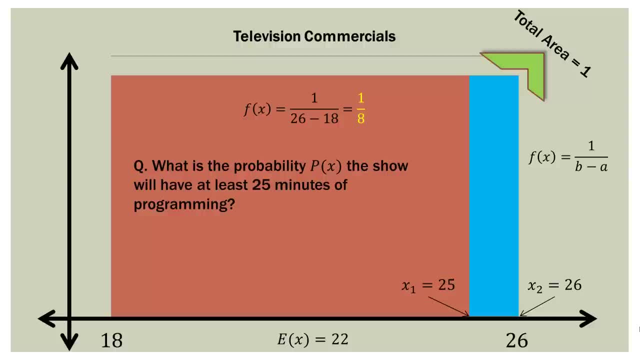 of our distribution. That's the area that represents at least 25 minutes of programming, the probability. Now, to do that, we use a very simple formula. We use this formula here: X two minus X, one, divided by B minus A, And that's simply a ratio. 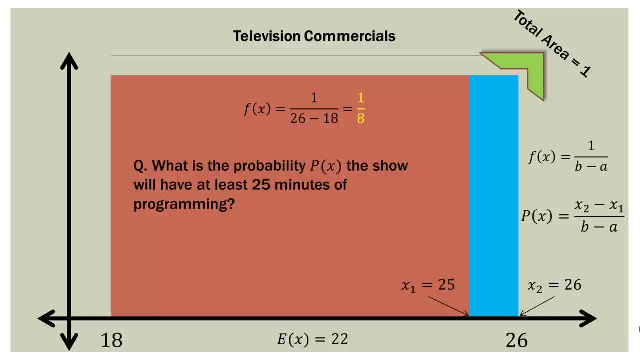 So the area of the blue as a part of the larger area there in the orange. So we go ahead and substitute those in. So X two is 26 minus 25, which is X one, which is one divided by 26 minus 18, which is B minus A. 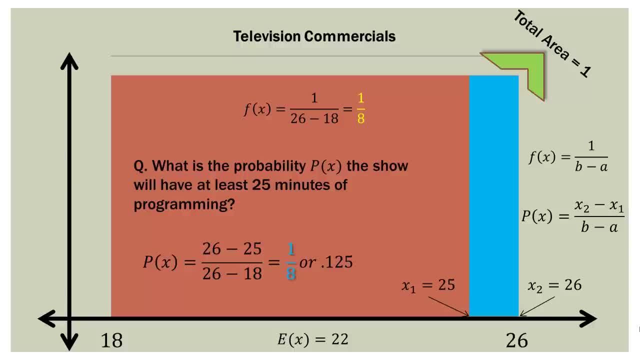 26 minus 18.. So that is one eighth or 0.125.. So the probability that a show will have at least 25 minutes of programming is 0.125 or 12.5%. So again, we're just finding the sliver. 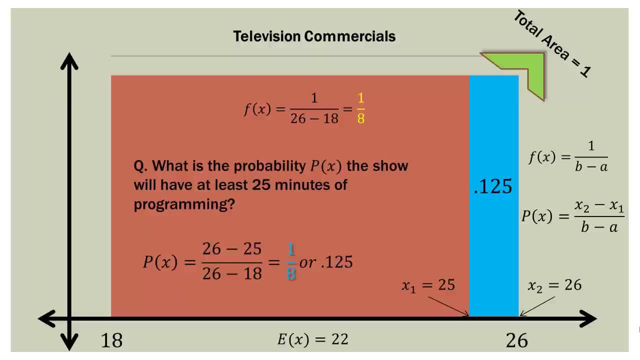 of our overall distribution. that's represented in our problem as a proportion of the overall probability of one So X, two minus X, one divided by B minus A. Next question: what is the probability the show will have between 21 and 25 minutes of programming? 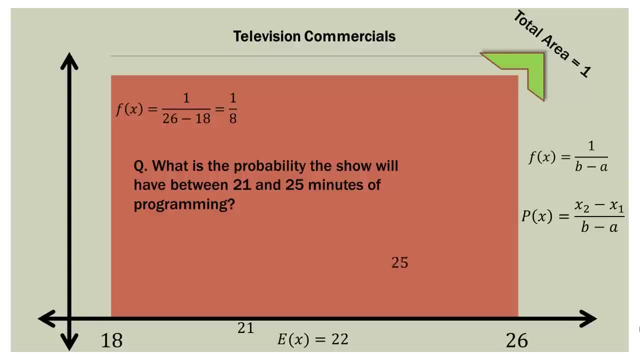 So we're interested in this part of the distribution that starts at 21 and ends at 25.. So we want to know the probability that is inside this blue region here. Now, of course, we can find that out using our probability function there on the right. 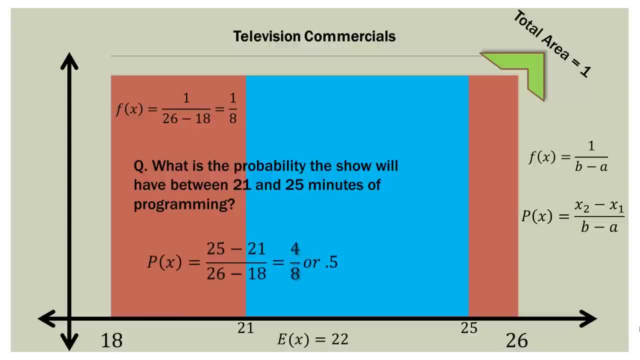 So X two is 25 minus X one, which was 21,. that's four divided by B minus A, which is always eight. so that's four over eight or 0.5.. So the probability that a show will have between 21. 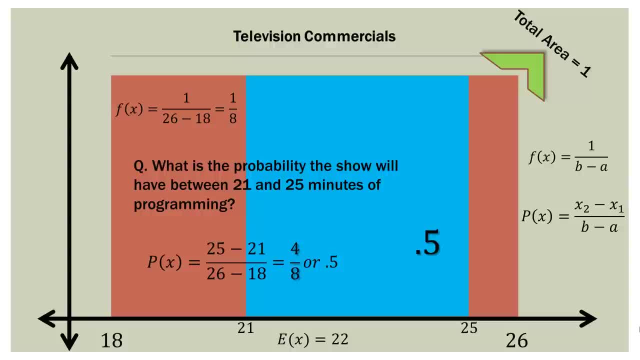 and 25 minutes of programming is 0.95.. is one half or .5.. And if you sort of look at our graph here it kind of makes sense That blue section looks like it's about half of the overall area there in the orange. 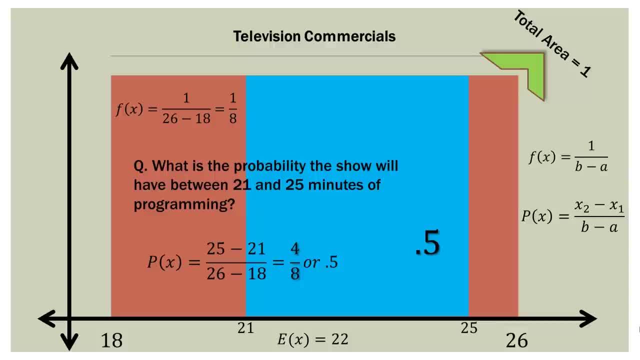 Now, I just eyeballed the 21 and 25, so it might not be perfect, but if we set up our rectangle there in the blue to be this big and we come up with an area that's like .1,, we probably wanna go back and look okay. 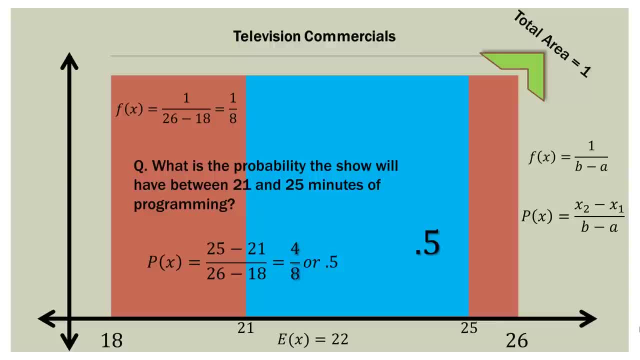 So we just use a lot of information to double-check our answer informally. So in this case it is .5.. Now what's the probability? the show will have between 22.32 and 24.77 minutes. Now here's where the continuous data. 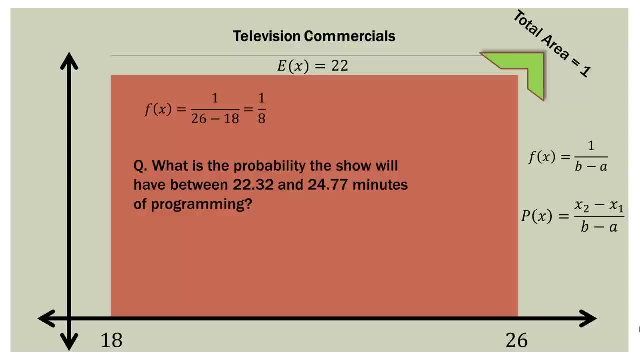 really comes into its own because remember that time can be measured to an extent that our instrument and instruments allow. So if we have a clock that can measure down to milliseconds, we can measure time all the way down to milliseconds. If we have an atomic clock, we can measure it down. 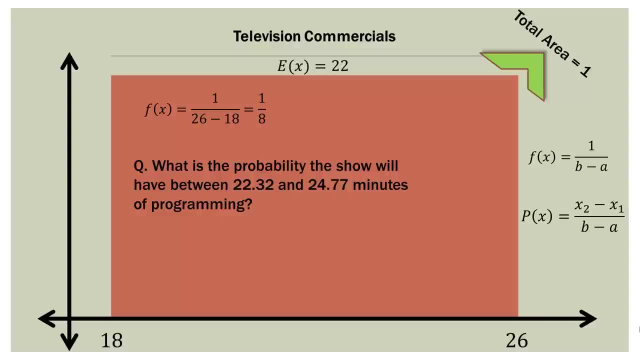 to some crazy number of digits, I'm sure. So our measure of time in this case is only limited by the precision of our instrument. Now compare that to the coin flip and the die roll. That's gonna be either heads or tails. 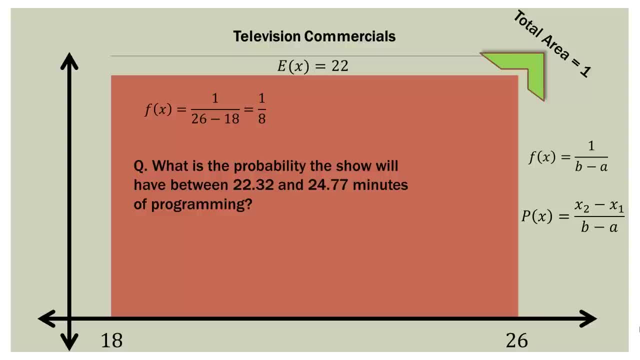 or one through six, no matter what, Where this, in this case time, is. simply. the measurement is simply limited by the precision of our instrument. So, theoretically, we could have the probability of 22.32356789 and 24.7756431.. 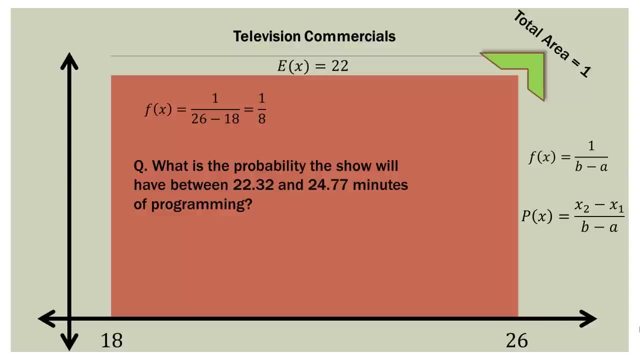 We could have that because it's continuous data. But since we're using this as a continuous distribution, we can actually go ahead and find this And we find it the exact same way. So we have 22.32 and 24.77,. 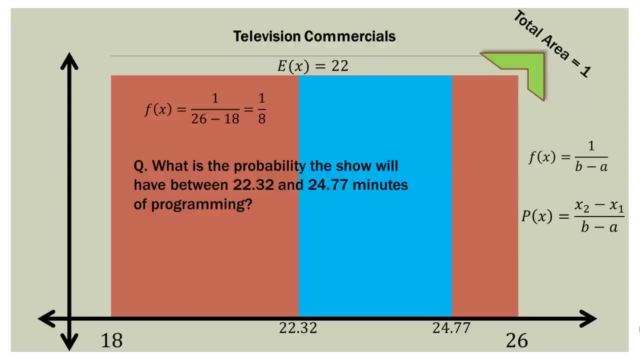 which is approximately this area in the graph. Now, before we actually figure out what it is, use some common sense to say approximately what area do you think this is going to be? Does it look like about half? Does it look about 1 tenth? 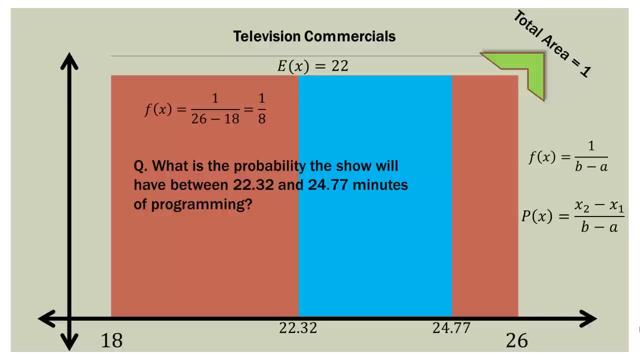 Does it look about .8 or 8 tenths? What does your common sense tell you? Well, to me it looks like it's probably not quite a half bigger than a quarter of it, So somewhere between a quarter and a half. 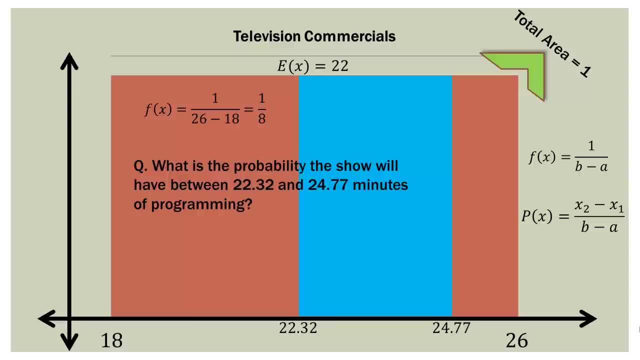 So we should have an answer somewhere in that range, just by our common sense alone. Now, when we go ahead and calculate it, we have 24.77,, which was x2,, minus 22.32,, which is x1,. 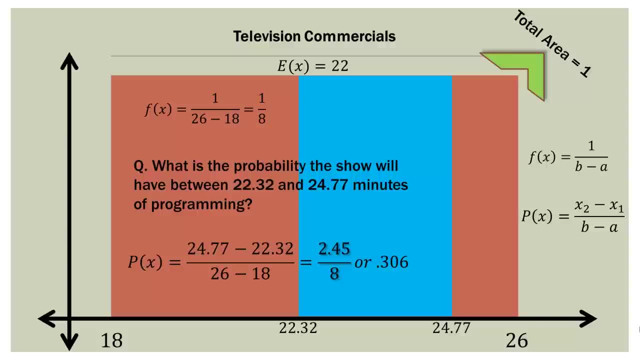 again divided by b minus a, which is 26, minus 18.. So that's 2.45 divided by eight or .306.. And that sort of made sense from our intuition. So the area there in the blue, which is the same thing as saying the probability, 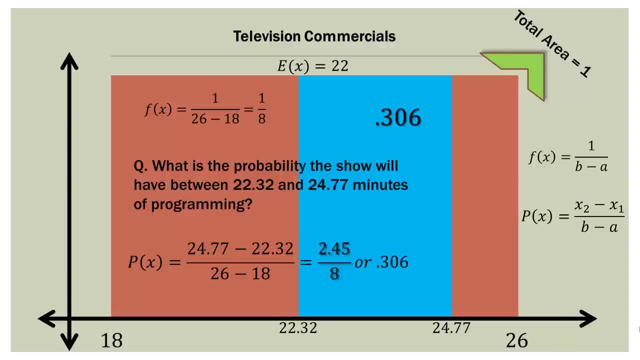 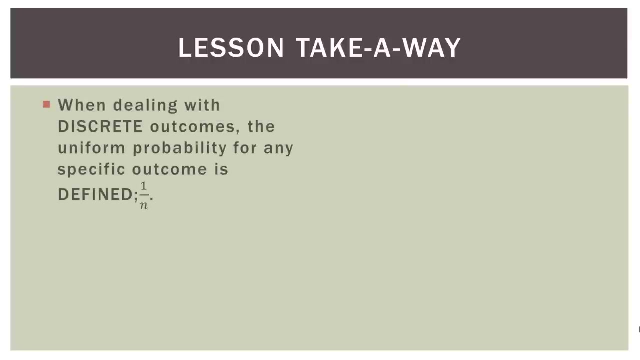 there in the blue is .306.. So the probability that the show will have between 22.32 and 24.77 minutes of programming is .306.. Okay, so a few lesson takeaways and then we're done When we're dealing with discrete outcomes. 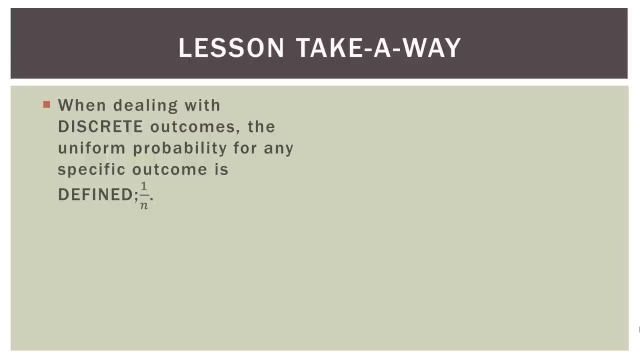 the uniform probability for any specific outcome is defined as one over n, where n is the number of outcomes. So for our coin flip, one over two, because we had two outcomes: .5.. Dierol was one divided by six, which was .167.. 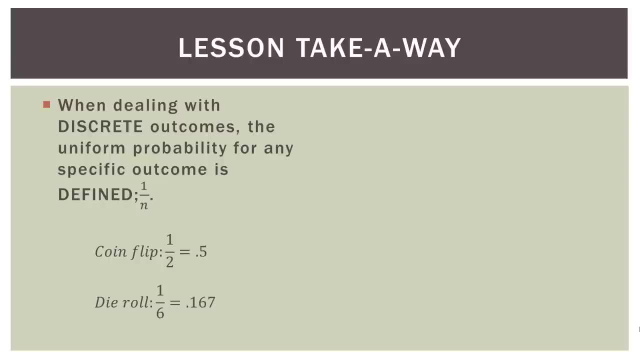 And that's because those are discrete outcomes. There cannot be any other outcome, And those outcomes, of course, are finite. Now, when we're dealing with continuous outcomes, like we did with the time, like we could do with measuring something's mass or whatever, 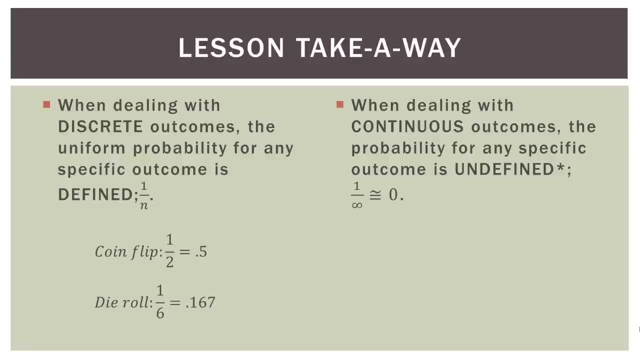 the probability for any specific outcome is actually undefined. So n is just extremely large. It's only limited by the precision of the instrument we're using to measure it. So one divided by infinity, .5.. Ncd is treated as zero, And because of that we can only find a range. 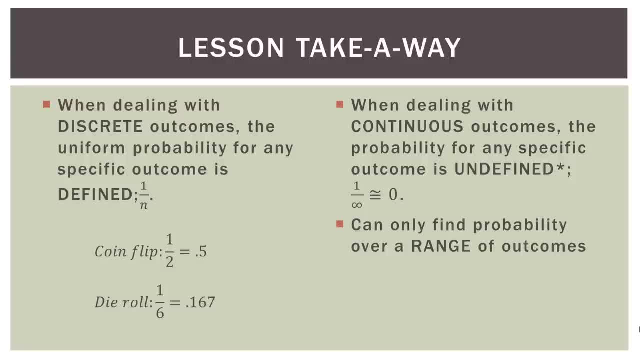 of the probability over a given range, not at a specific outcome. Now, what we're doing here- just for the purists out there and those that are interested- what we're saying here is that as n approaches infinity, okay, it approaches the limit of infinity. 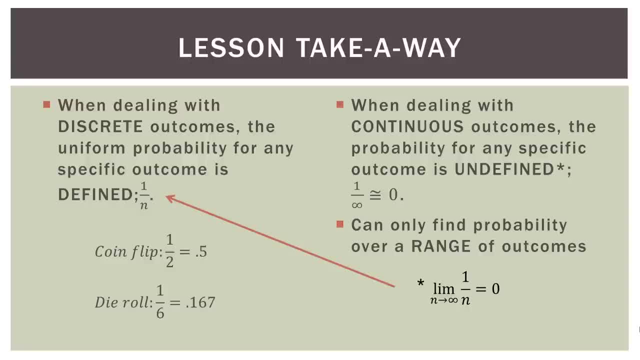 is that is being treated as zero. So that's where this zero concept comes from, because one, over an increasingly high number, just becomes infinitely small. so it's sort of a limit problem. if you wanna know Now in everyday words that I use with my students. 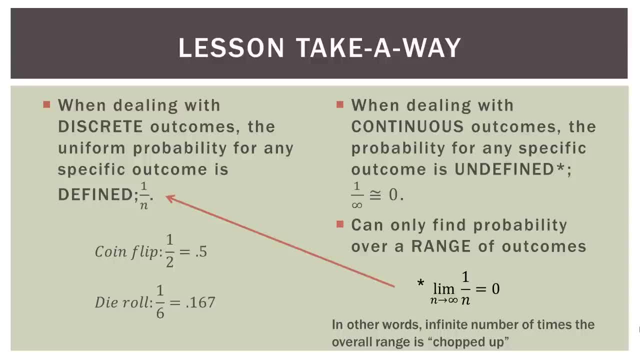 in other words, the infinite number of times the overall probability, the overall range is being chopped up. So for the die throw, we chopped it up six even times. For the coin flip, we chopped it into two even pieces. For the bus stop, we chopped it into 10 even pieces. 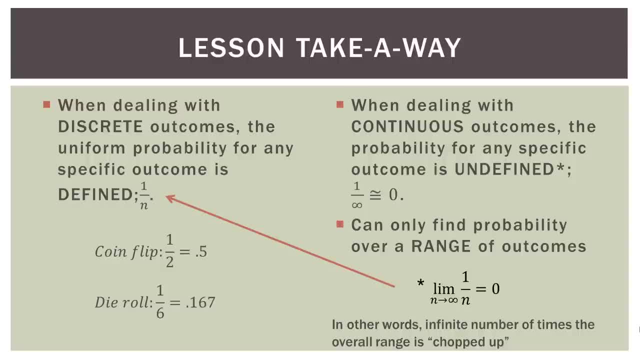 But if I were measuring time to four decimal places, think of how many times I would have to chop that up in the very, very, very, very slim bits. It's basically an infinite amount, And the probability of any one of those is so small it's practically 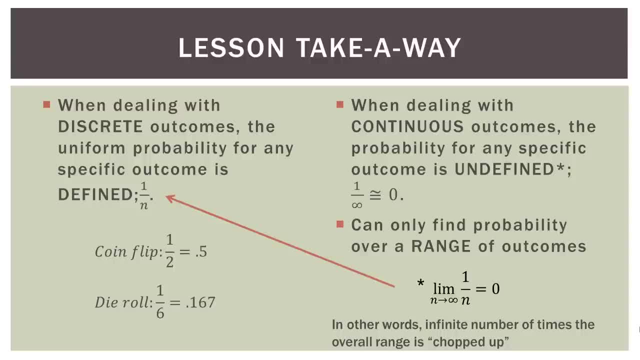 zero. So that's really the difference here. Discrete is one over n, where n is a relatively moderate number, like two, six, 10, something like that. Continuous is as n approaches infinity, And that's again where we treat most of our measurements.